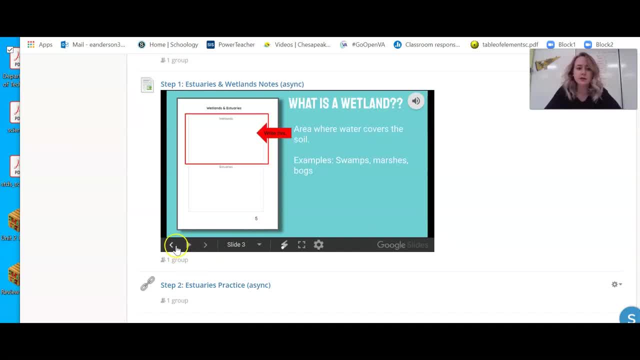 and it'll take you to the electronic version. Today we're talking about estuaries and wetlands. Let's fill this out. What is a wetland? A wetland? you could tell by the name. it's an area where water covers the soil. It's wet, So examples are swamps, marshes and bogs. 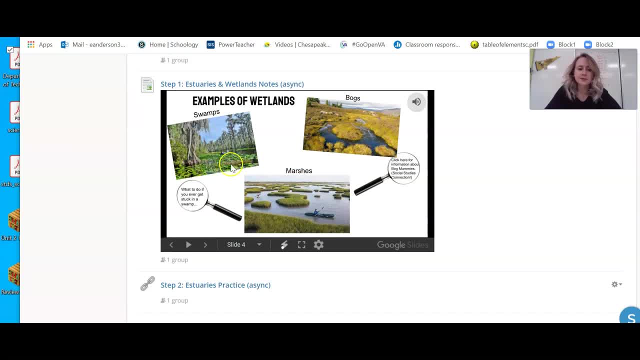 Write that down there And again. here are three examples of wetlands And if you want to click for more information, you can do that. Here's an example: Social Studies Connection, bog bodies, for instance, and stuff. Wetlands or bogs are very good at. 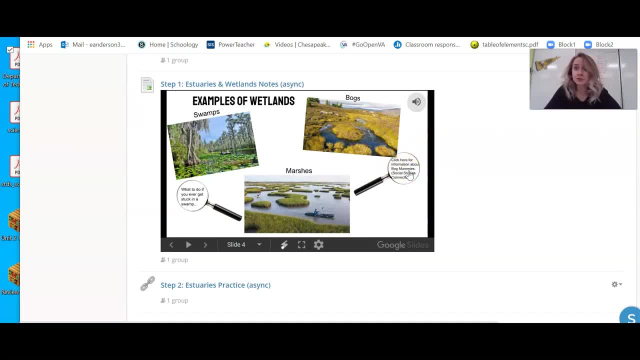 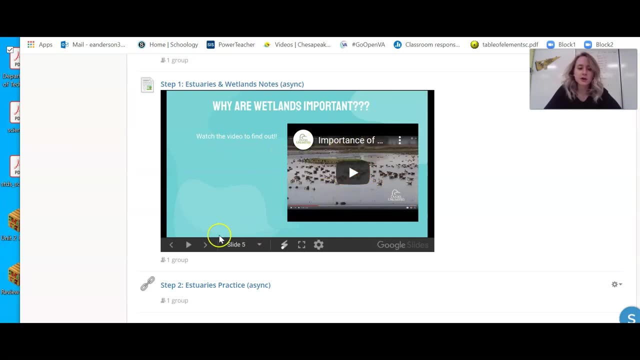 preserving human humans. So if you get buried in a bog, you become a mummy. So anyway, that's a cool connection. And then what to do if you're ever stuck in a swamp? Why are wetlands important? Watch the video to find out. So you're going to pause this video. watch that video. 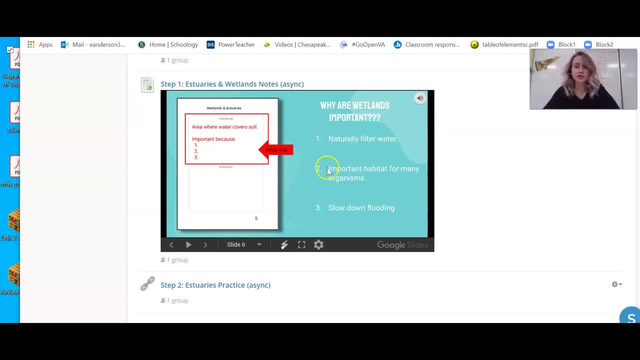 and then let's fill this in. So there's three reasons wetlands are important: They filter out the water, They're a really important habitat and they slow down flooding. So now we're going to go to the bottom parts of the notes. What's an estuary? An estuary is a place where the fresh 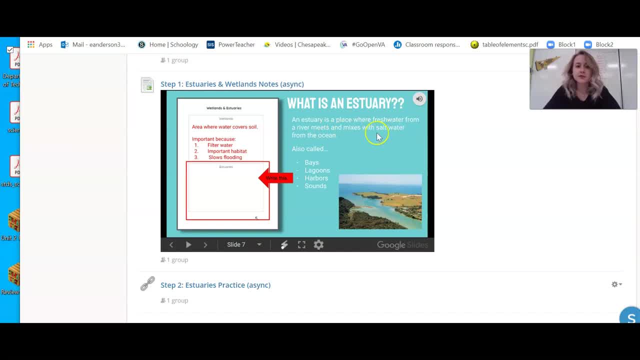 water from a river is mixing with the salt water from an ocean, So this happens at a river's mouth, right? That's our vocab word. They're also called bays, lagoons, harbors, sounds. An example is the Chesapeake Bay, So just write example. 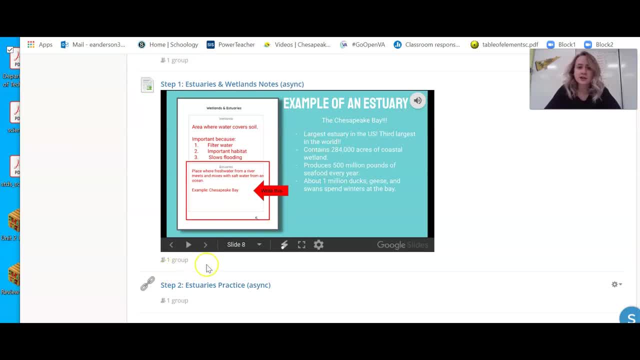 Chesapeake Bay. This is the largest estuary in the US, third largest in the world, and it's a really important place for creatures to live. It's an important habitat and it's important because it produces a lot of the seafood that we eat. 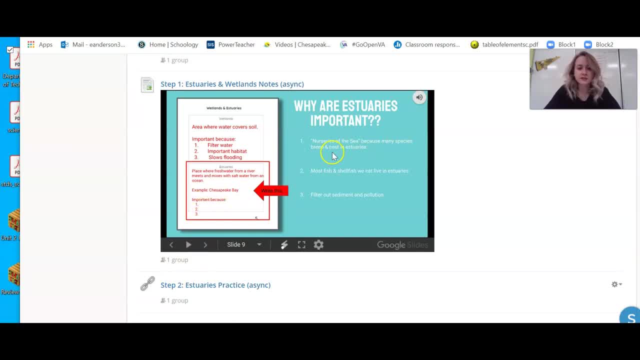 Estuaries are important because three reasons, and let's write this down: They're called nurseries of the seas. Many species nest and they breed in estuaries. Most fish and shellfish we eat come from estuaries and they also filter out sediments and pollution. So make sure you write. 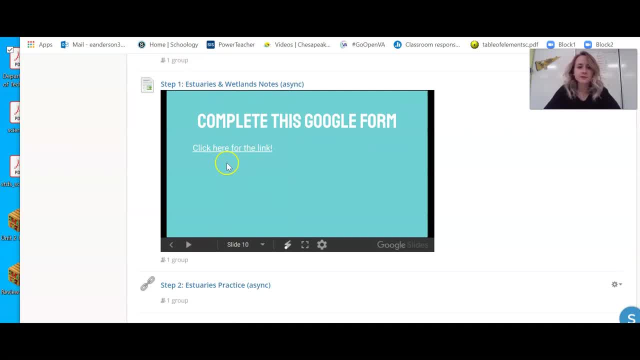 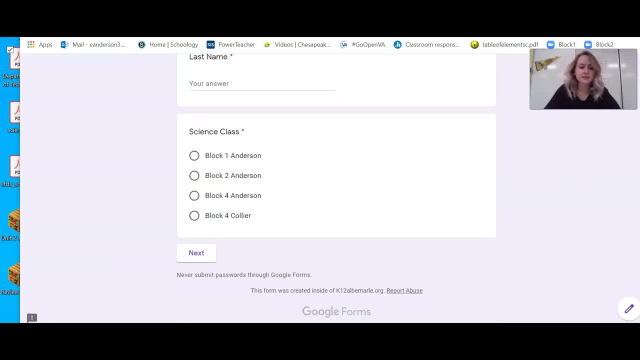 those three down And then the next thing you're going to do is complete this Google form. So you're going to click here and this is what you're going to do. You're going to write your first name, last name, science class, and then click next. Bodies of water where fresh water from streams.